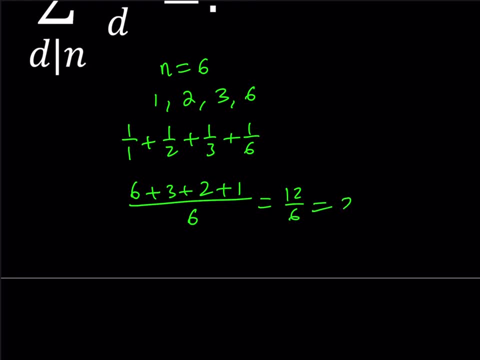 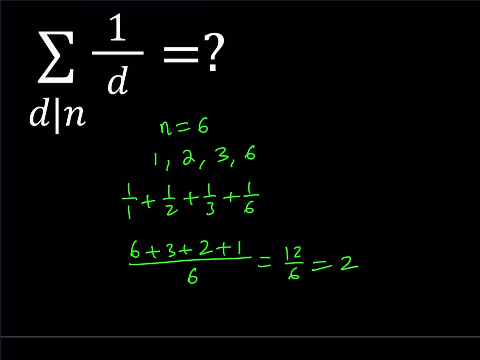 12 divided by 6. And in this case it just happens to be a 2.. Okay, you can take another example and just keep working with this, But let's go ahead and continue. So in this problem, I'm trying to find 1 over d And notice that in this case I wrote the divisors in numerical. 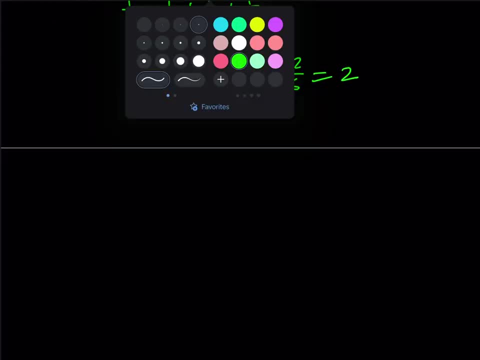 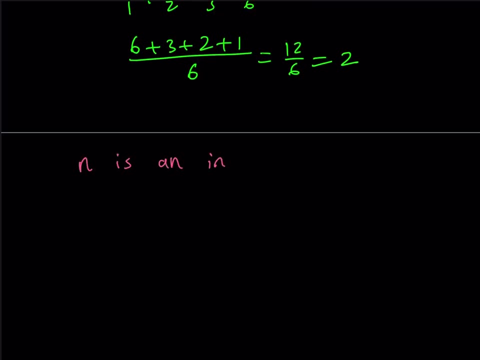 order. So I'm going to be doing the same thing in the general case as well. So that's why it's important. Okay, so suppose n is an integer And let its divisors be d1,, d2,, dot, dot, dot all the way up to dk, where k is the number of. 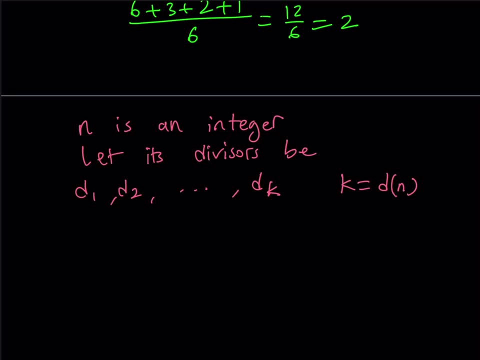 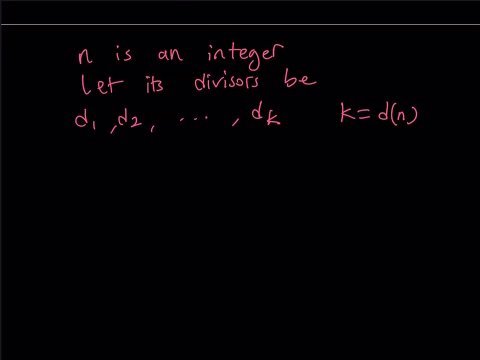 divisors of n. Remember, we use d of n for that purpose. So these are all the divisors of n, k, divisors of n, And I want to make sure that these are all in numerical order. That's important, pairing them and pairing them up. So it's important that they are arranged from smallest to 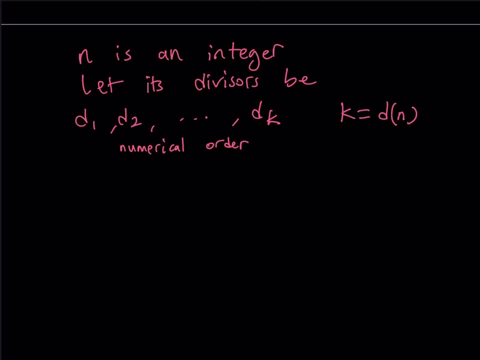 largest. Obviously, the smallest divisor would be 1 in this case, and the largest divisor would be the number n itself. Okay, so now we're going to go ahead and add the reciprocals of these divisors. Let's go ahead and write that down as a sum without the sigma 1 over d1 plus 1 over d2,. 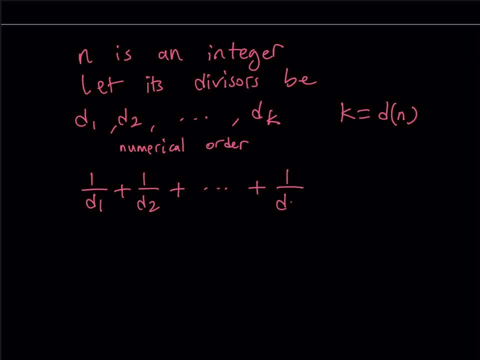 dot, dot, dot, and it's going to end with 1 over d2.. Again, I'm not writing these as is, but d1 is 1 and dk is n, So let's go ahead and write that down: d1 is, the smallest divisor is 1, and the largest divisor is the number itself. But that doesn't. 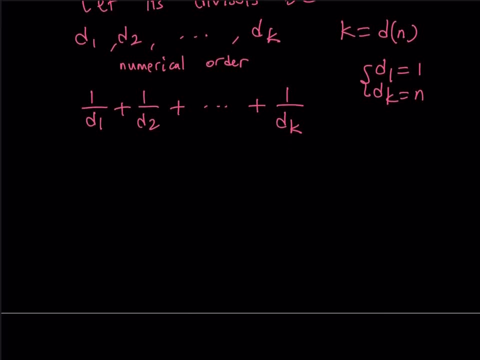 matter, because we're going to solve this in the general case. Okay, so what am I going to do here? Well, you can make a common denominator. Obviously, that's one method to look at it, but I'm going to be using a slightly different approach. Pretty much the same thing, but 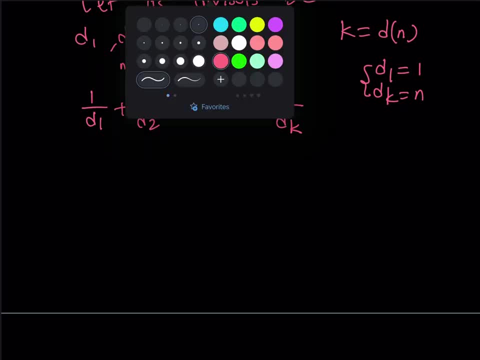 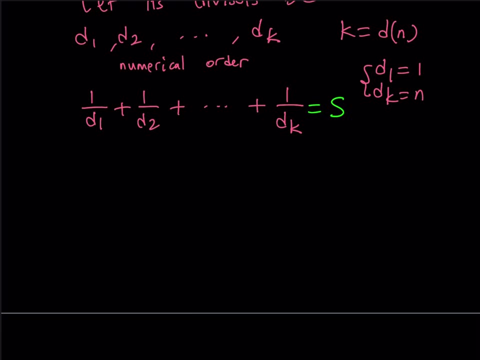 it's kind of more fun to do. So, this sum that I'm trying to calculate, I'm going to call that s, which makes sense, right, Because it's a sum, It's not a product. So, and then, after this, 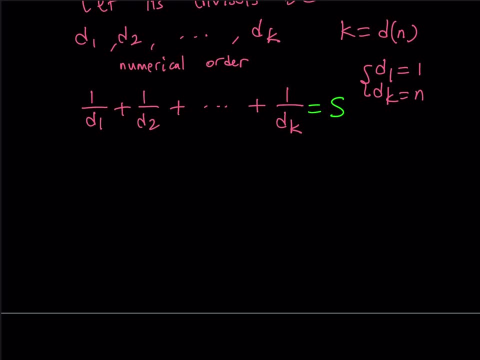 I'm going to multiply. This step is actually critical. I'm going to multiply both sides by n. Multiply by n. And why am I doing this? You're going to know in a little bit. So when I multiply both sides by n, obviously I have a sum on the left-hand side. So every term, 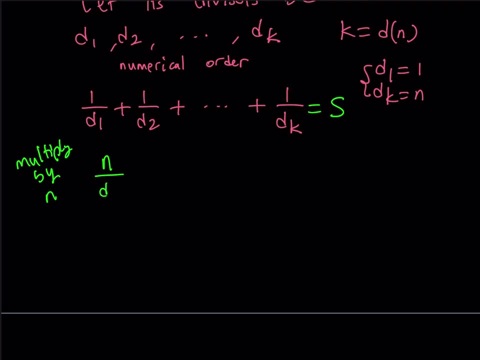 in the sum will be multiplied by n, So it's going to look like n over d1 plus 1 over d2.. n over d1, n over d2, dot, dot, dot. n over d of k is equal to n times s. Now notice that. 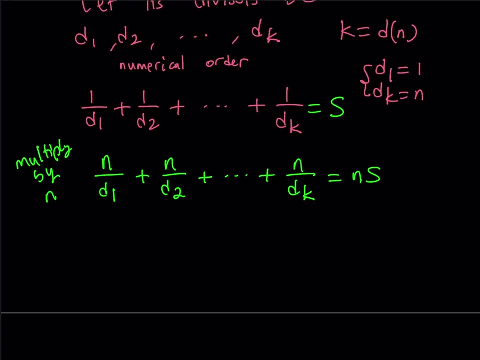 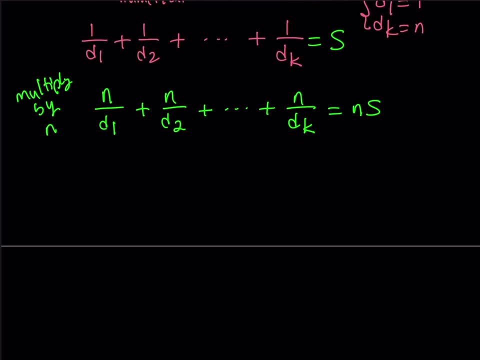 d of k is d sub k is equal to n, So the last one is going to be 1, and the first one is going to be n. So we're basically adding all the divisors right, Or the sum of the, or we're adding 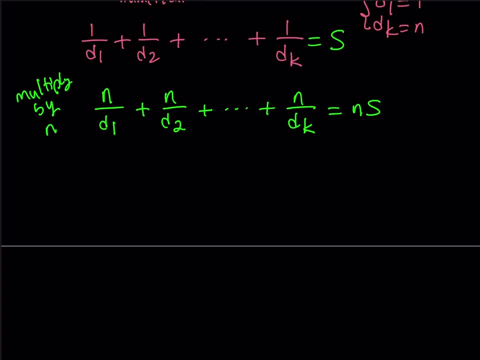 wait, did I say divisors? We're not adding divisors. We're adding the reciprocals of the divisors. But guess what? We're adding the divisors. So we're adding the divisors. So we're adding the divisors. But we said that at the beginning we're going to put them in numerical. 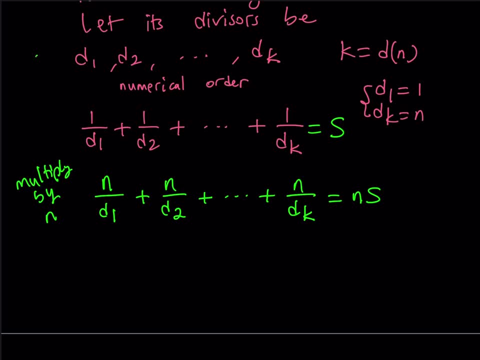 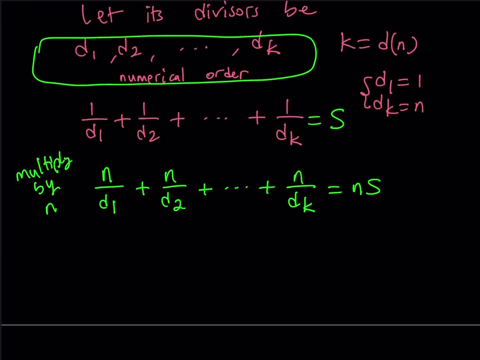 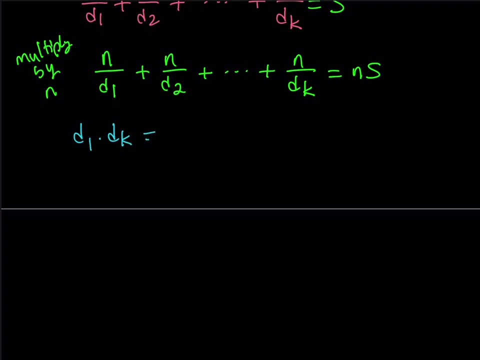 order. So what is that sum supposed to represent, right? So let's take a look at this list here. This means that since the smallest one is d1 and the largest one is dk, when I pair them up, I can kind of write it like this: d1 times dk, which is 1 times n, by the way, is equal to n. 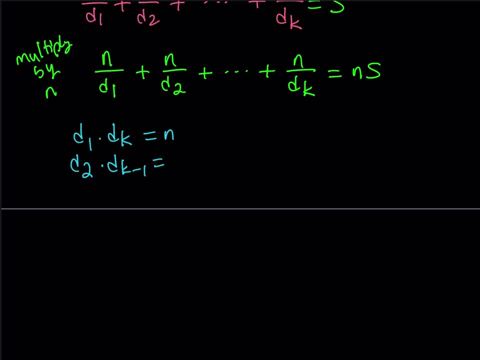 And the next one, d2 times dk minus 1, is also going to be n. Now think about the case of 6, right, 1, 2, 3, 6. You pair them up like this and the product is always equal to n right. And then this is going. 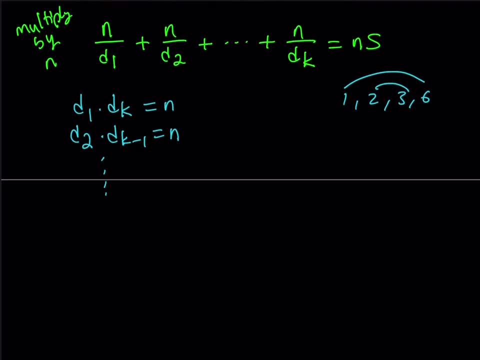 to continue, of course, all the way up to what You're going to continue, And what that's supposed to mean is that, for example, if you divide n by d1, you're going to get dk, Or if you divide both. 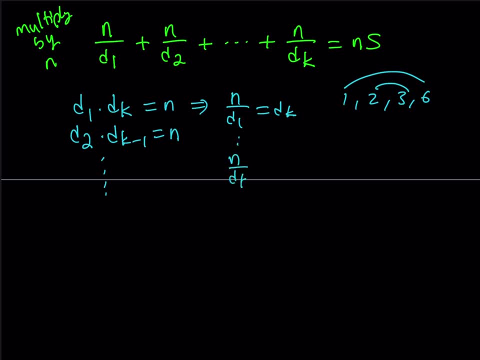 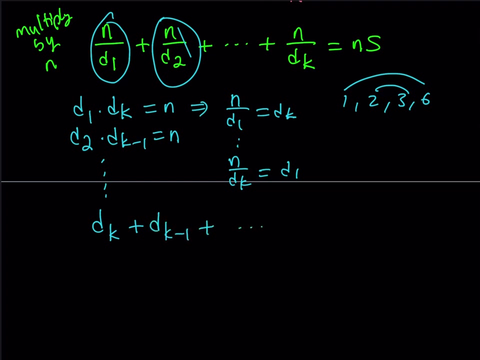 sides by dk, you're going to get n over. dk is equal to d1.. Wow, that's interesting. So this basically equals d. This one is equal to d Oopsies. This one is equal to d sub k minus 1, dot, dot, dot And at. 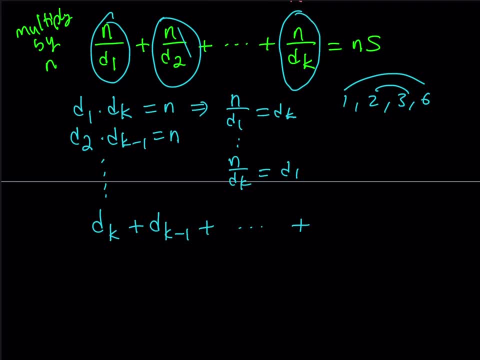 the end, n over d sub k is going to equal d1.. And what is that supposed to mean? Well, we kind of got the sum of the divisors, but in reverse order. Pretty much the same thing, right? So this is the.